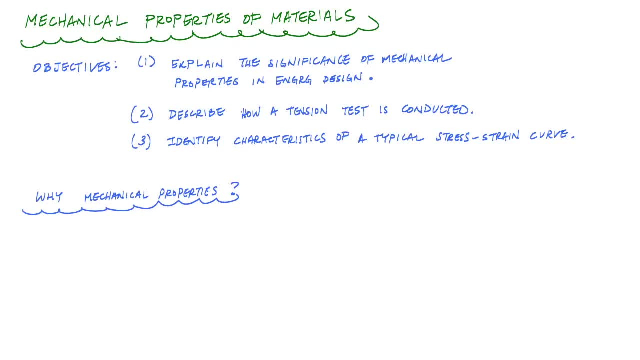 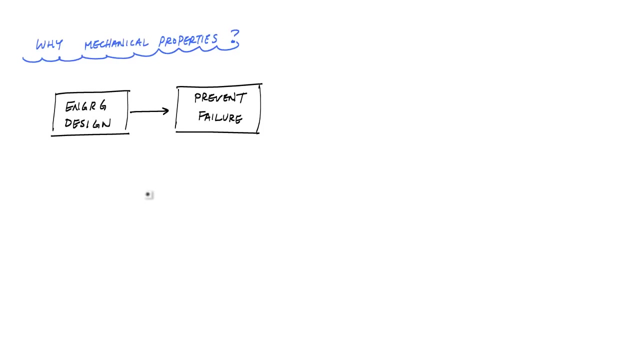 Now, generally speaking, the reason we need mechanical properties is because we want to be able to design stuff, And engineering design is largely associated with trying to prevent things from failing, Like, for instance, how much weight or force can I apply on a bridge before it collapses, Or how many people can I fit in an elevator before the cables snap. 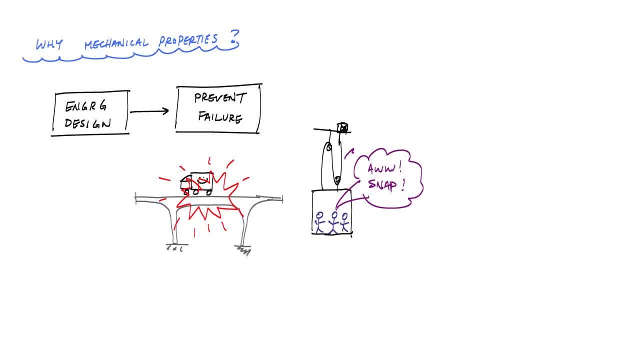 In general. you could look at a lot of stuff around you right now, And the reason that it is the way it is is so that it doesn't break when you use it And that you know if it's durable. it lasts a long time, it can survive all the loads that you apply to it. you think it's a good design. 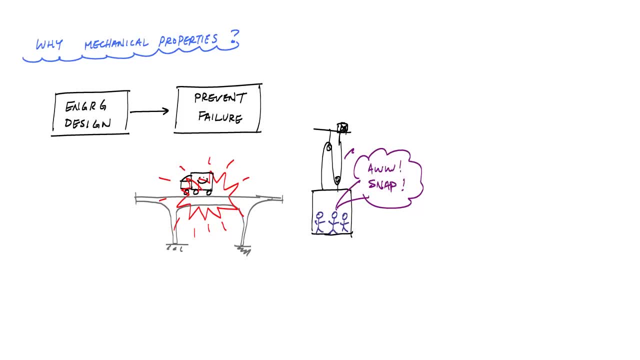 Now we take all of these cases of where something could fail and we define them mathematically by their stresses: The stresses that occurs in the material. And because there's only two types of stresses, most of the time we can just say that what we want is in our designs. we would like the applied normal stress to be less than or equal to whatever we allow. 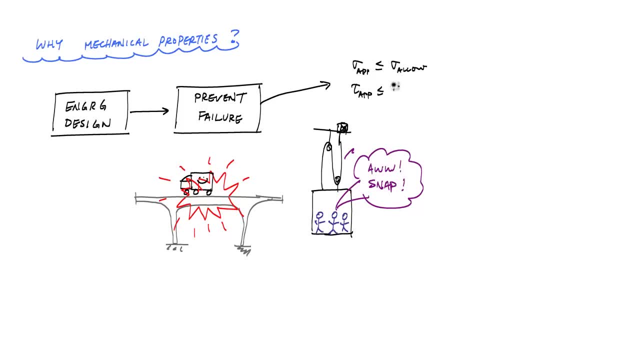 And we would like the applied shear stress to be less than whatever we allow Now in order to put limits on what we define as safe or what. here we have to define what is considered failure And this sigma allow. these allowable stresses that we, as engineers, choose are a way for us to define. 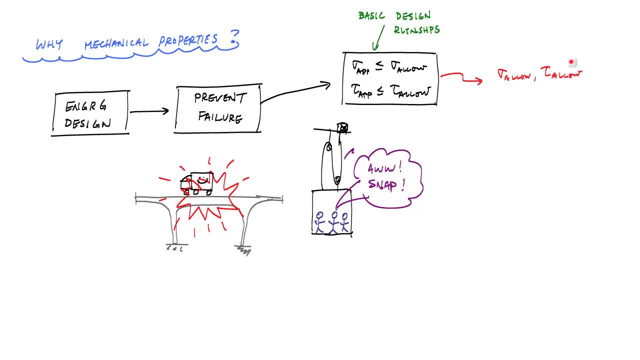 how, if or when something fails. And in order for us to define these components, these allowable stresses, you know, we have to have an understanding of how the material behaves, that we choose and how it fails. But for us to figure out when the material fails, we need to do a stinking experiment. 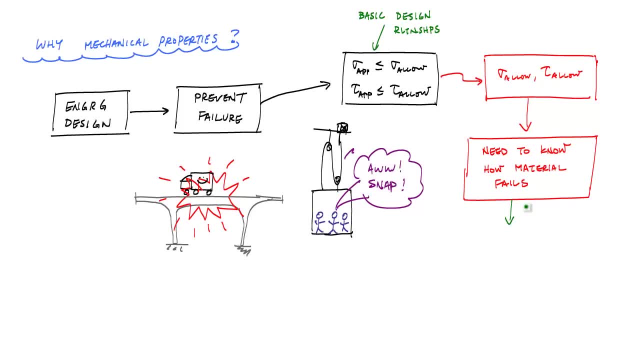 All right, And really that experiment. all you need to know is really take a piece of material and break it apart, Right? You know how many times have you done that already before you've, before you've had a sense of whether or not it can hold it. 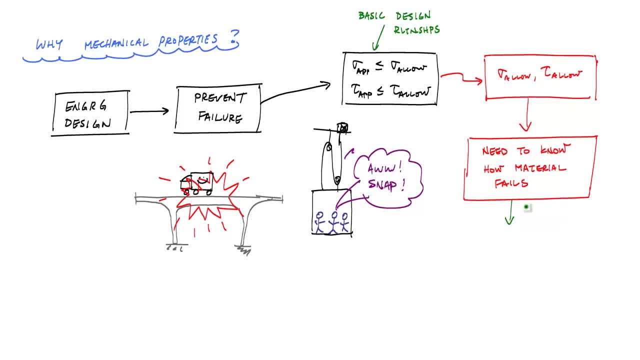 you had a touch. You know, bend it. bend it like buying a shoe. you know is the shoe going to be comfortable? so you bend it and it's all flexible, and you're like, oh yes, very flexible. And so, bam, you buy it. 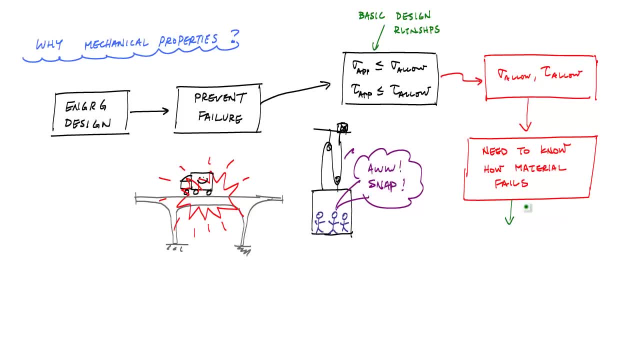 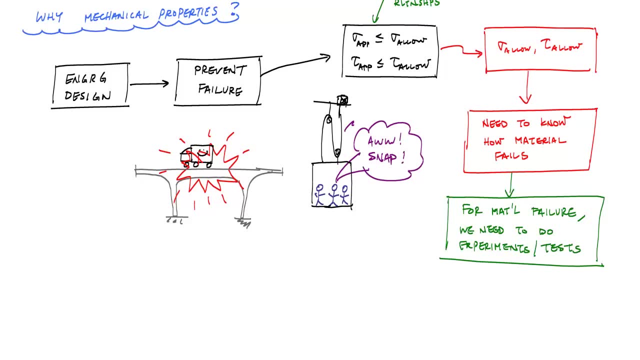 So we, as engineers, want to do this with actual numbers. We want to actually quantify material failure. So now we want to do these experiments and tests so that we can determine the stress at which something breaks, or, you know, the most stress that a material can handle. 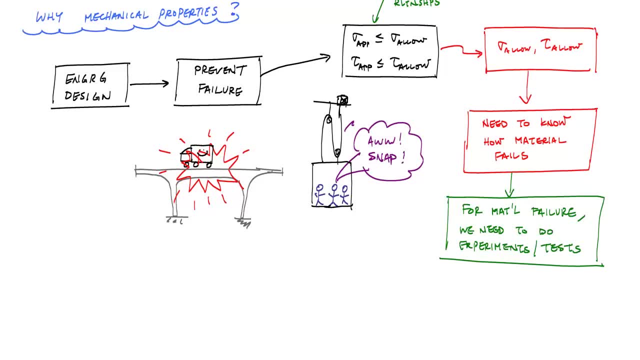 And the most common experiment to do- that is what is called- is what is called a tension test, And the tension test is exactly what it sounds like. It's like taking a material and just pulling it apart, And there are machines that are built specifically to pull and compress material so that you can break stuff. 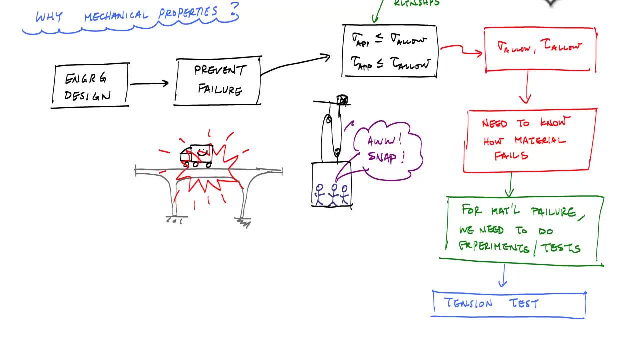 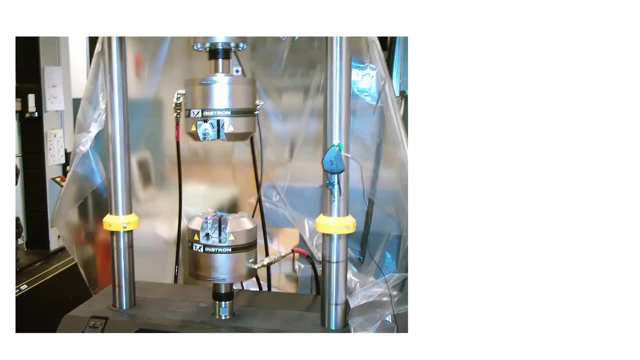 you know, to do an actual test, And they cost hundreds of thousands of dollars, And what you're looking at here is a servo hydraulic actuator. who's really the real function here is just to move this head up and down, back and forth, so that you can pull apart or push and crush materials that you're going to put inside these grips. 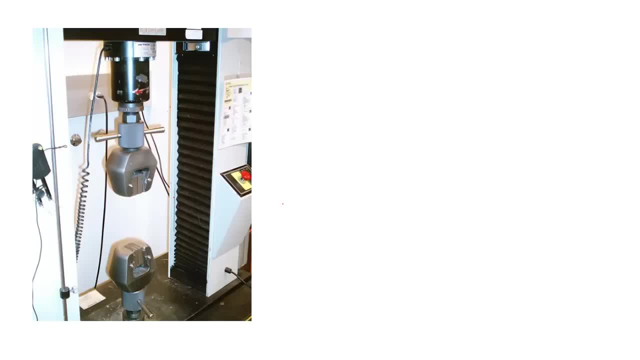 This is a picture of another device, the same type, you know, same idea, But this one is electromechanical. It doesn't need fluid pressure to provide the force to pull apart materials. But here you can see like hand tightening grip. 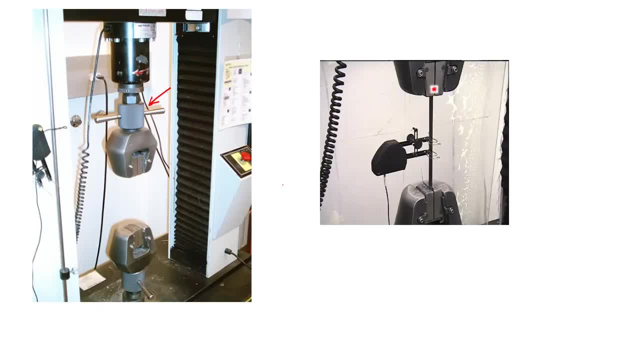 And here's a picture with a carbon composite specimen put inside for a tension test. And then you can see the extensometer right here clipped at these two points. And what the extensometer does is measures the deformation program it to divide by the original length between these two clips. 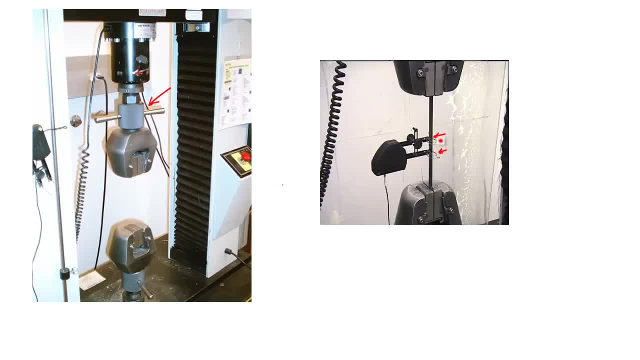 And it'll give you a measure of the normal strain that's occurring within the specimen. And over here there's a force transducer And that force transducer measures the amount of force that the actuator is applying, And then you can calculate the stress by dividing by the area. 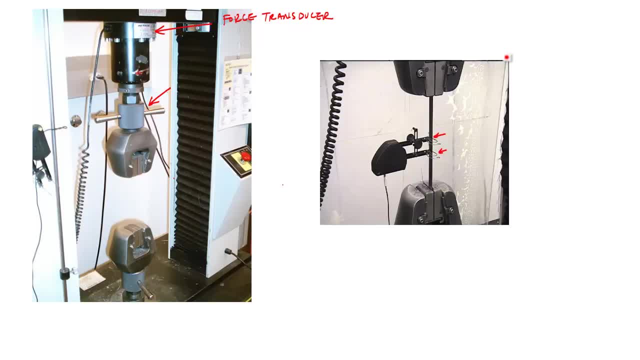 And this is all you know- set up into some sort of data acquisition system, So it'll make measurements every second or whatever, every five seconds or every half second, however fast you know the processing can work, And then eventually the specimen will look like this for a carbon composite: 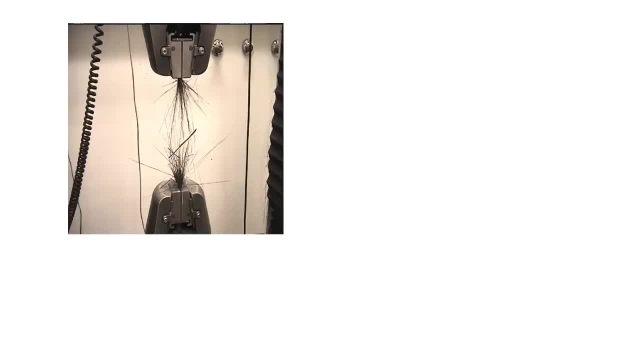 This one was a protruded carbon composite specimen- And really all the individual fibers go bing, bing, bing, bing, bing, bing, bing and then boom, the whole thing breaks. It's pretty crazy. 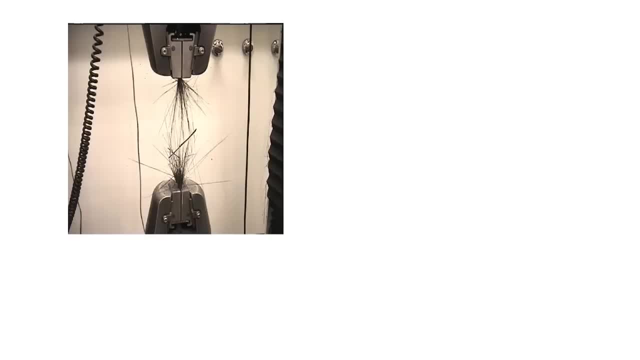 Fiber's shooting everywhere. It's kind of dangerous. You got to put some like plexiglass in front and behind Just to make sure that the fibers wouldn't come out and shoot and hit people. Most common material that we want to at least get introduced to and be familiar with is steel. 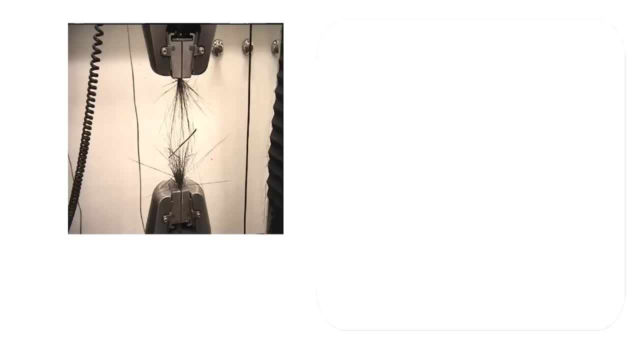 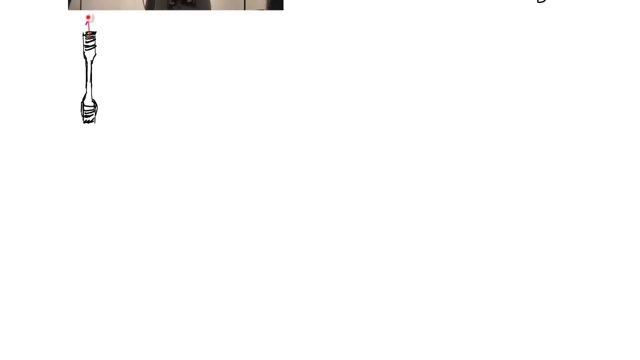 Steel is a very popular material to use in lots of structural applications And so the stress strain cover steel. you can watch- There's a bunch of YouTube videos. The stress strain test of steel typically involves taking a steel specimen. It's put into the tension testing machine, grabbed at the ends and pulled apart. 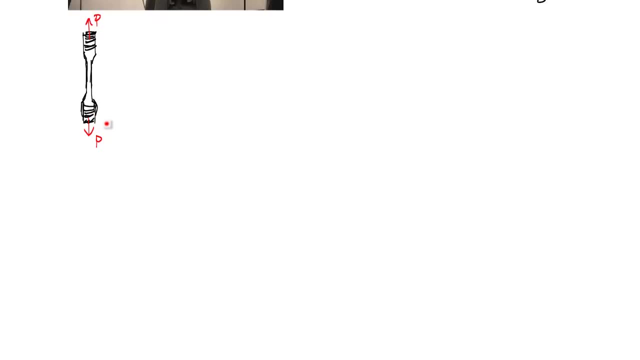 And you're going to again take data measurements. You're going to calculate the deformation, You're going to calculate the stress And you're going to be able to plot the stress strain curve. And the stress strain curve for steel looks something like this: 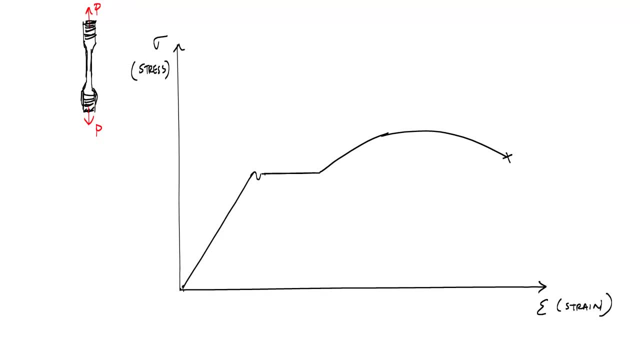 So this isn't drawn to scale, But it's exaggerated so that we can identify different regions And I can write them down here all in one drawing. When we do a stress strain test for a steel specimen, what we have is this first portion. 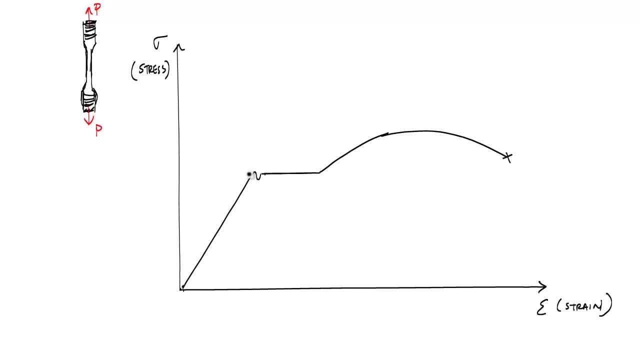 right here, from zero load to some increasing load, We have what is called the linear elastic region, which is a straight line, right, Linear, It's a line, And this is called the linear elastic region, which means that it behaves in this region. 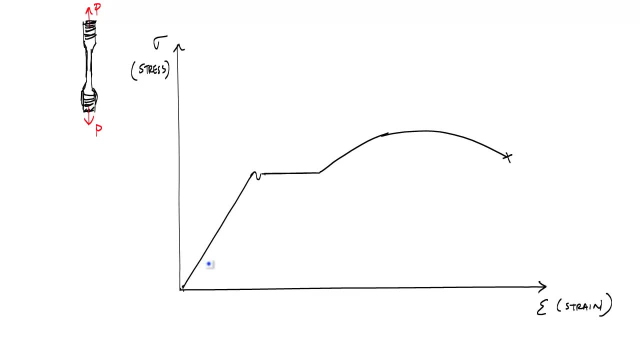 like a rubber band. You can load it and unload it, and it's supposed to return back to its original shape Once we get to this point right here, this is what we call the yield point, And I've drawn here what is an upper and lower yield point. 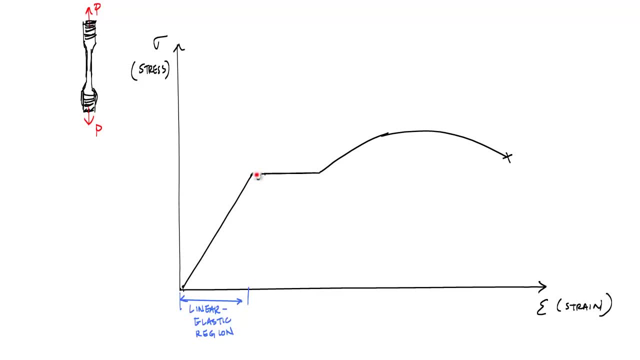 I think it's enough in mechanics of materials just to know that when you get, you move out of the linear elastic region, that that means you've yielded or you've become non-linear. And this is called sigma y, the yield stress. And when, once you've reached this yield point, or what time is it? sometimes it's called 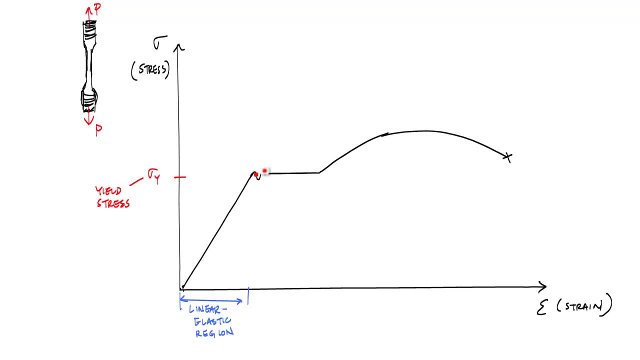 the proportional limit, you start to have permanent deformation. It's like bending a piece of plastic and it won't go back to its original shape. There's a point where you've you bend it just enough and in this region right here, where the loading stays constant but the specimen continues to elongate, is called the plastic. 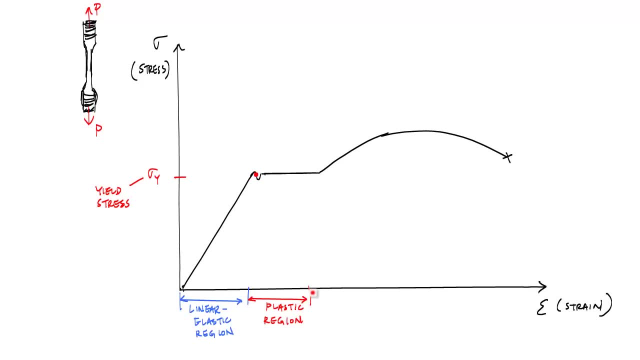 region. Then it seems like the material gets stuck, It's tougher or harder all of a sudden, you know, outside of this plastic region, And somehow it's able to start taking more load again and the load increases. thus the stress increases, until you reach a peak way over here, some peak value which we'll put. 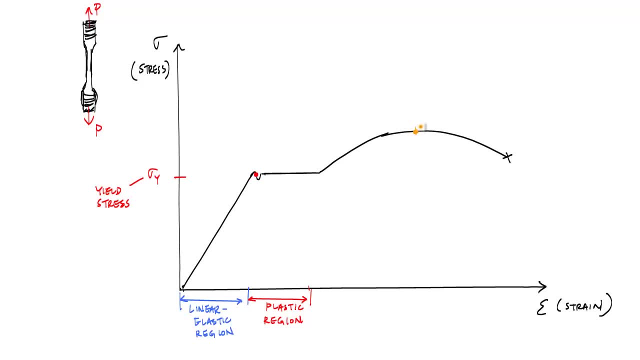 boom right here, the maximum or highest point on this curve. This is the ultimate tensile strength And people call this region up to the ultimate tensile strength. They call this the strain hardening region And if you talk to a material scientist they'll say that it's where you have. you've got way. 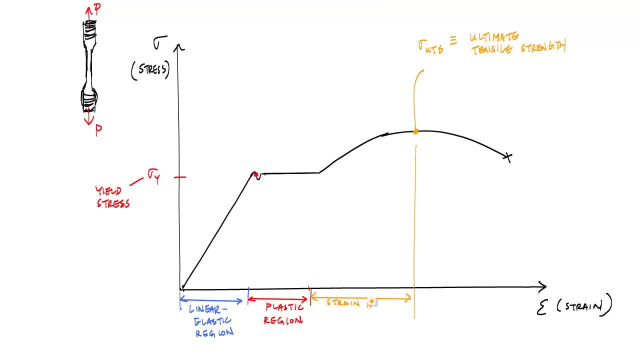 too many dislocations and there's no more room left for dislocations, and so the material is able to take on more load and reach this ultimate tensile strength. Another way to look at it is like kind of like all the grains and everything lined up. 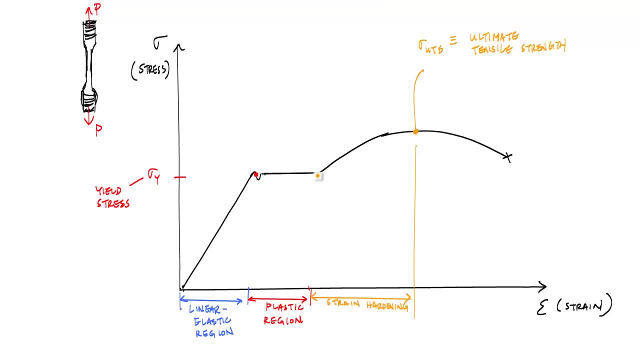 you know just right as you were in this plastic region And then all of a sudden it was all lined up And just holding down as much as it could, and now the load starts increasing here And then finally up to failure and you get to a point. after you reach this, it starts. 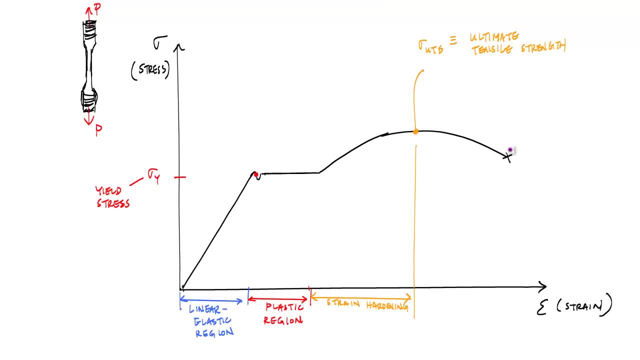 decreasing again the stress that's going on. And here is where we get fracture, sigma fracture, And this would be called the fracture strain, where the specimen physically breaks And this region. what happens is You will see a noticeable thinning out of this region, right here. 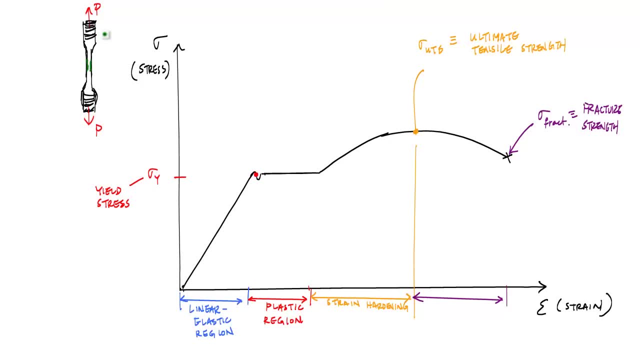 You will start seeing it kind of stretch and become really, really thin, So the cross-sectional area will get really, really small. It might look something like getting really thin right here, like a neck, And you will see that this is called. this is called the necking region. 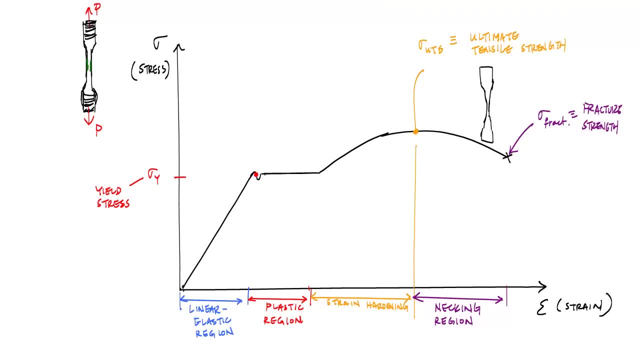 And the values that are really important, or at least the ones that are used the most often in structural steel design, Are the ultimate tensile strength, the yield strength or yield stress, and then the slope of the linear elastic region, which is called the modulus of elasticity or Young's modulus. 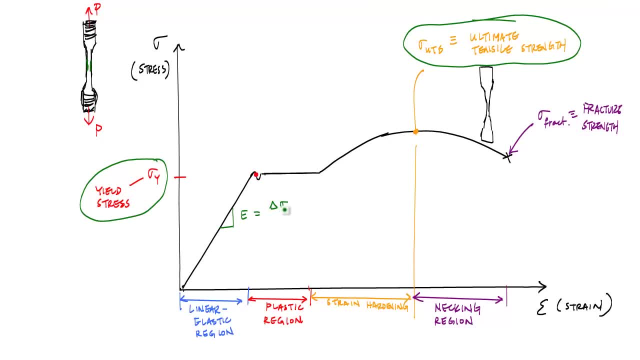 And it's just simple slope calculation. So it would be like change in sigma over the change in strain or rise over run. Now, as part of an allowable stress design approach, when you define the allowable stress, this sigma fail over the safety factor. 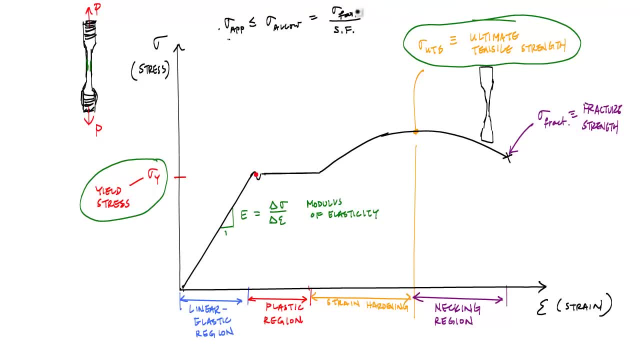 This sigma fail might be Depending on the application. it could be the ultimate tensile strength, It could be the yield strength of the material And then the safety factor typically is prescribed by codes In general with the first course in mechanics of materials. all the equations that we use. 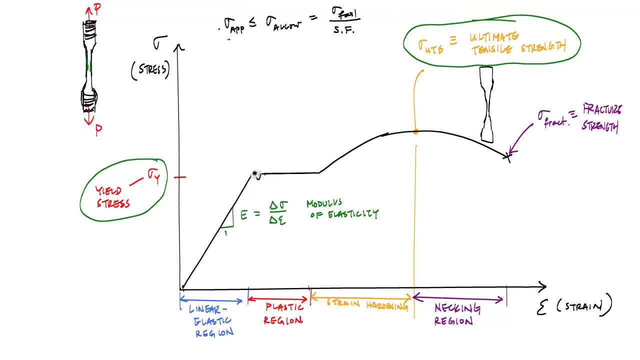 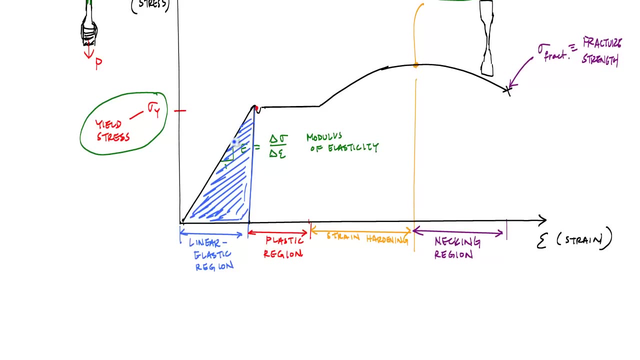 are assuming that we have a linear elastic material. So for the most part, everything that we do in our material state, we are in this linear elastic region. Another very important aspect of Of this linear elastic region is that here. here is where the linear relationship between 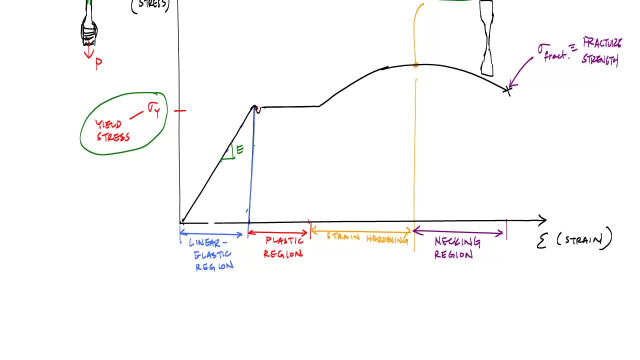 stress and strain was observed by Robert Hooke way back in the day, And this relationship, sigma E, sigma, or this normal stress, is equal to the modulus of elasticity times the normal strain, And this is 1D or one-dimensional Hooke's law. 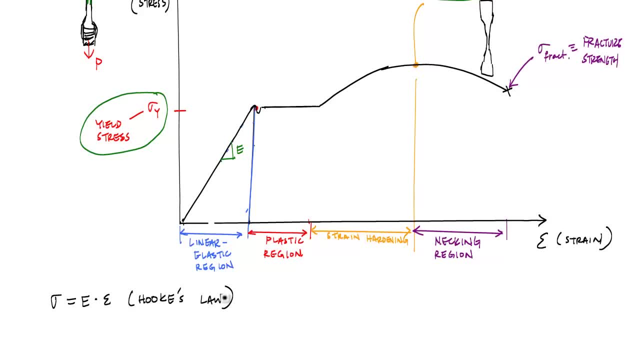 And this is really important. This is something you should remember for the rest of your life. You know what I'm saying. It's like that important And I, You know, to make me remember, I always think of, like Captain Hooke. 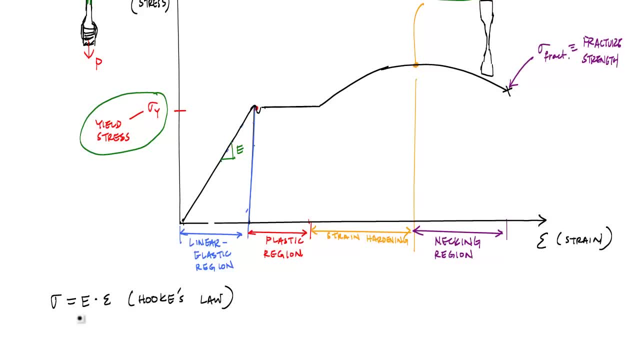 Arrgh, Right, Like a pirate Arrgh. Anyway, And just to give you a sense of the modulus of elasticity: this Young's modulus for steel is 29,000 KSI For something like carbon fiber, like a high modulus carbon fiber. this could be somewhere. 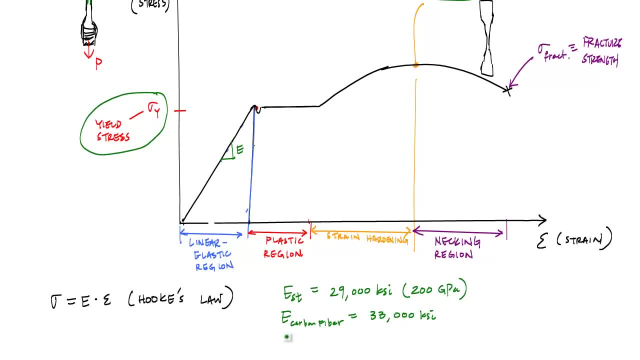 around 33,000 KSI. And then concrete is around. The typical concrete would be around 3,600 KSI And if you look at it, wow, you know we're talking steel and carbon fiber being about 10 times stiffer than concrete. 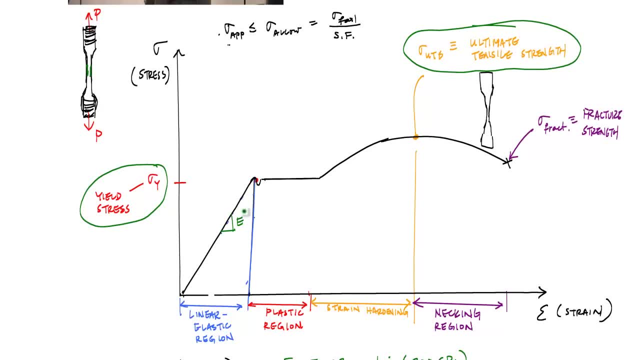 Another way to look at the stress-strain curve is to look at kind of the area underneath And if you look at the area, the area is like a measure of energy that it takes to break the specimen And so some cool or interesting properties, in particular because we're talking about, 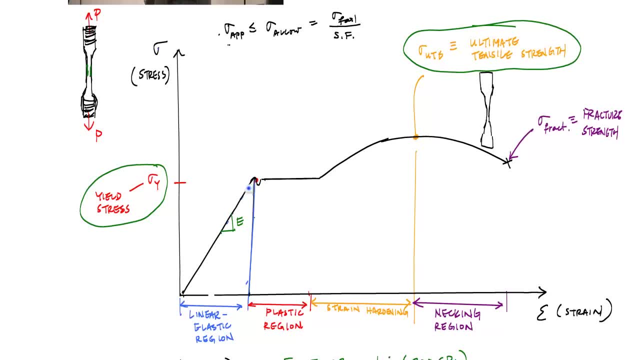 stress and strain. here we call that strain energy. But the amount of strain energy it takes to yield the specimen is this area here And this area is called the modulus of resilience. And you would just literally calculate this: It's a triangle, so one half base times height.